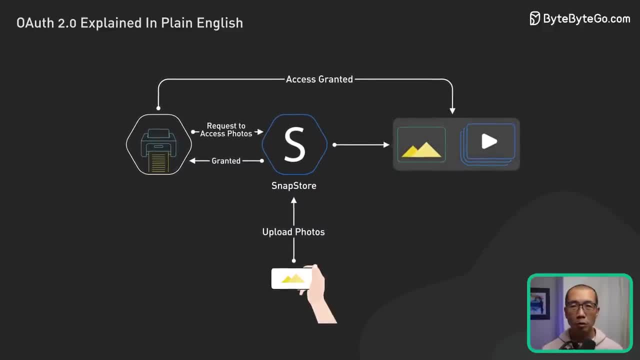 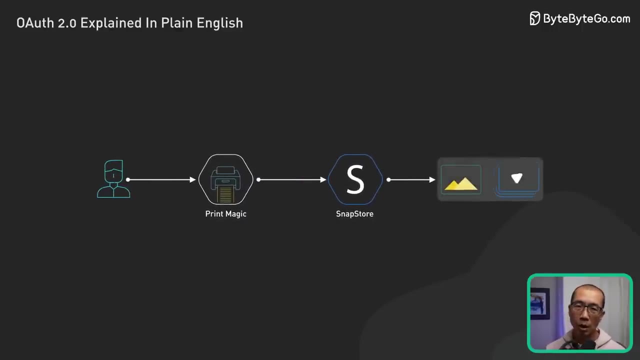 we grant PrintMagic permission to access our photos on SnapStore Using OAuth 2, PrintMagic can then access our SnapStore photos on our behalf without ever knowing our SnapStore login credentials. This is an example of the OAuth flow. It's an elegant stance between us, PrintMagic and SnapStore, all orchestrated by OAuth 2.. 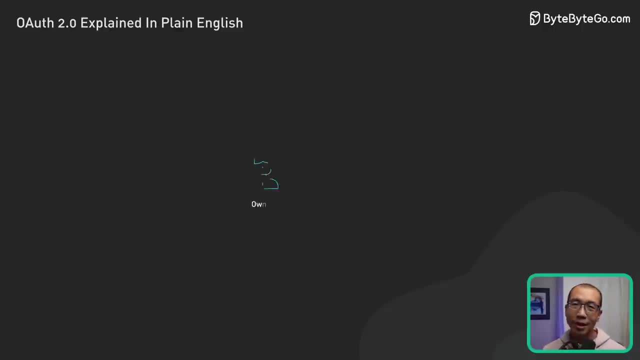 Now let's unpack this further. In this context, we are the resource owner, because we own our photos. is the resource server that stores our photos. Pre-magic is the client that wants to access the photos. The authorization server could be a part of SnapStore. 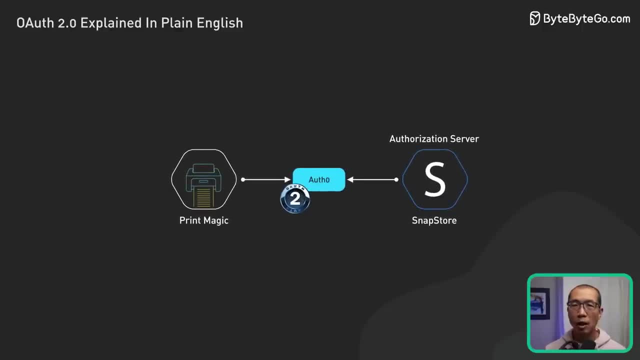 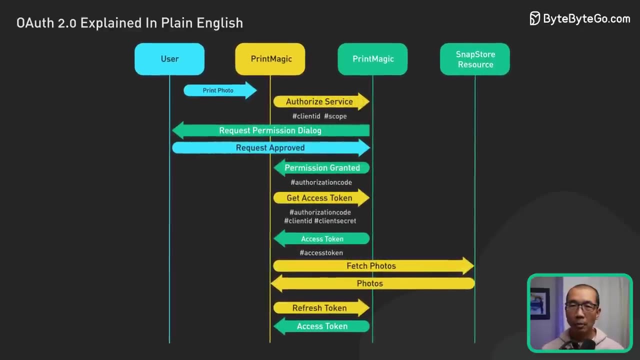 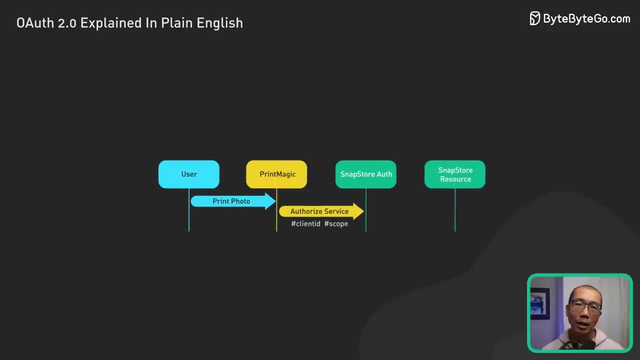 or an external identity provider and is responsible for handling the OAuth2 process. Let's follow the OAuth2 flow in this scenario. It begins when we instruct Pre-magic to fetch photos from SnapStore. Pre-magic sends a client ID and scope, which represent the access level requested. 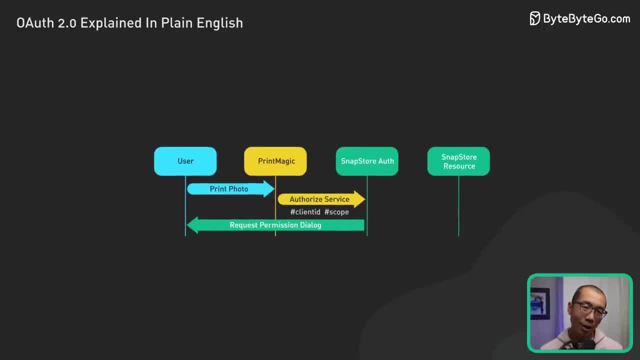 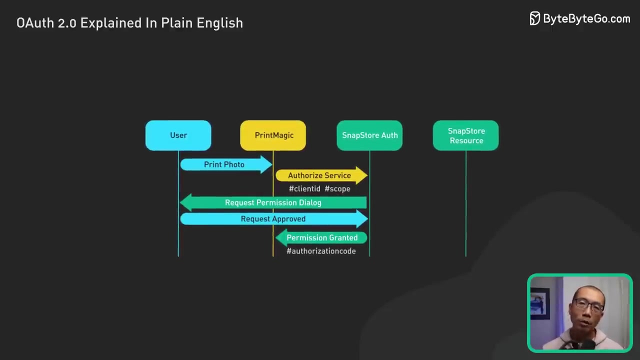 to SnapStore's authorization server. As the resource owner, we authenticate directly with SnapStore and grant Pre-magic the consent to access our photos. Once consent is granted, the authorization server sends an authorization code back to Pre-magic. Pre-magic then presents this authorization code. 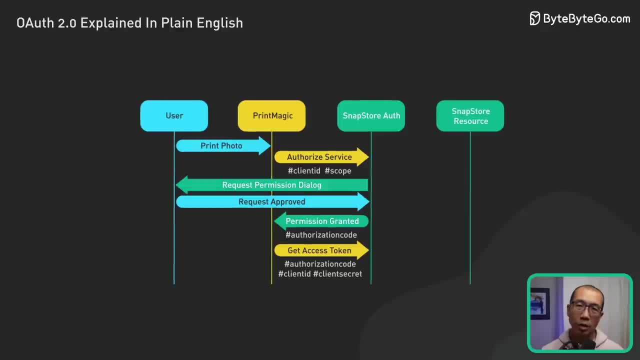 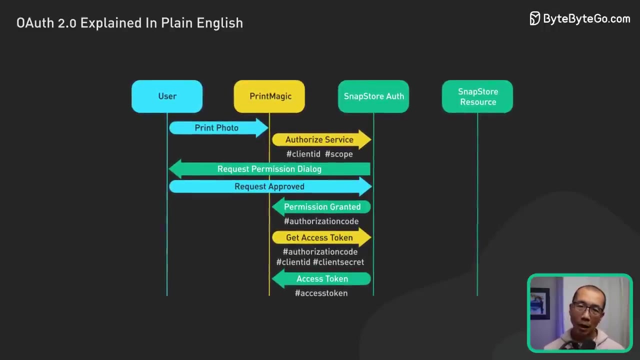 its client ID and client secret to the authorization server. The client secret is a private key shared only between Pre-magic and the authorization server. If the authorization server verifies the authorization code, client ID and client secret, it issues an access token to Pre-magic. 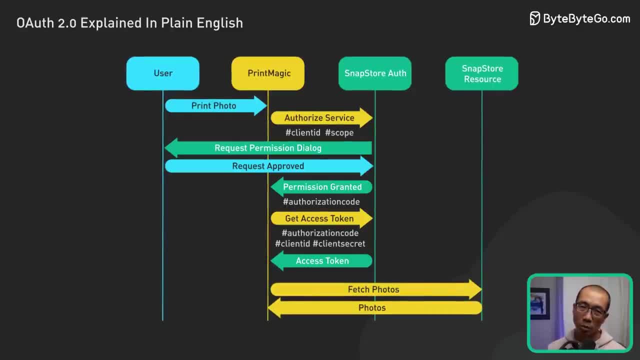 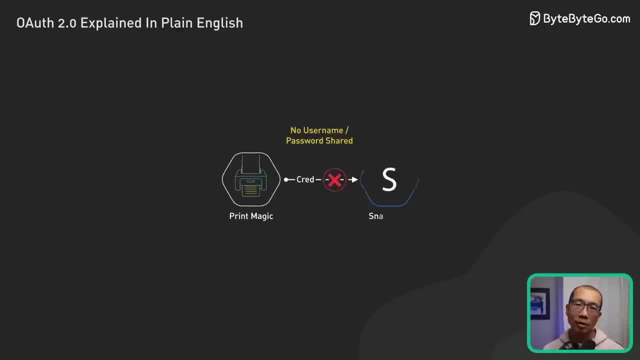 Finally, Pre-magic uses this access token to request our photos from SnapStore's resource server. This OAuth2 process ensures that our SnapStore login credentials are never exposed to Pre-magic, while allowing Pre-magic to access only the photos we authorized it to see.